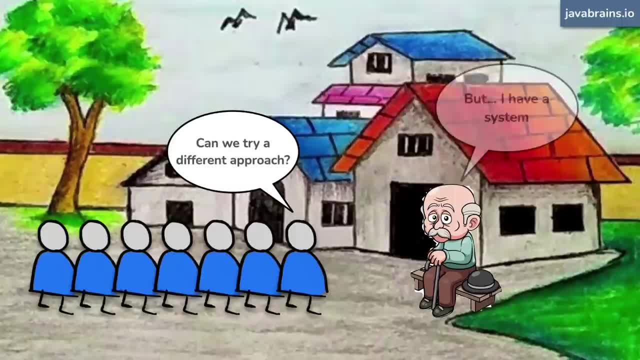 a different way for them to buy provisions, but the old man didn't want to hear any of it. He kept saying: this is my system, This is how I've been doing this for years and I don't want to change it. The people wished there was someone who could help them. 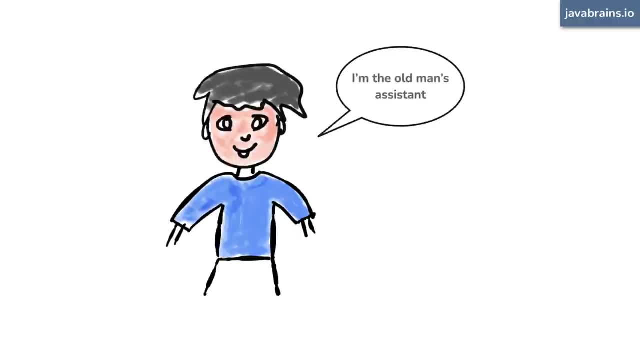 So there happened to be this village boy who worked as an assistant to the old man. His job was to help the old man as well as manage the line of villagers outside the shop. He would see the people in the village stand in line for hours and struggle, So he wanted to do something to help. 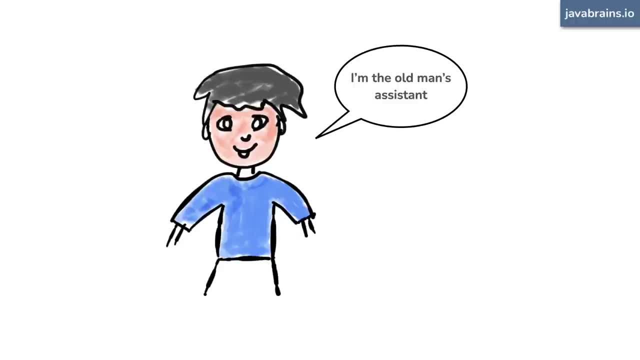 them while at the same time not having the old man change anything in the way he has been operating for so many years. He could very easily devise a system where the village folks could stay at home until it was their turn to gather the provisions, You know some kind of a token system or something. 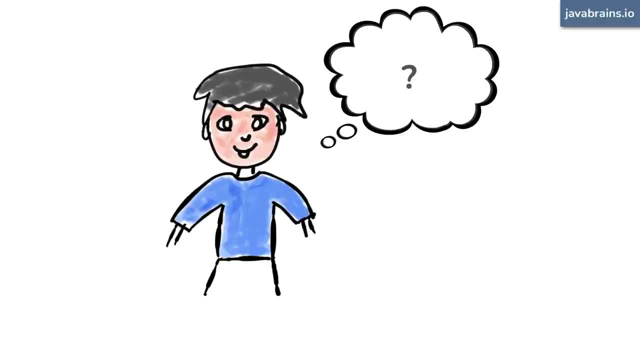 like that. But how would he implement something like this without the old man having to change anything, or preferably even knowing anything about it? One day he came up with an idea. He went to the old man and said: well, you know how. 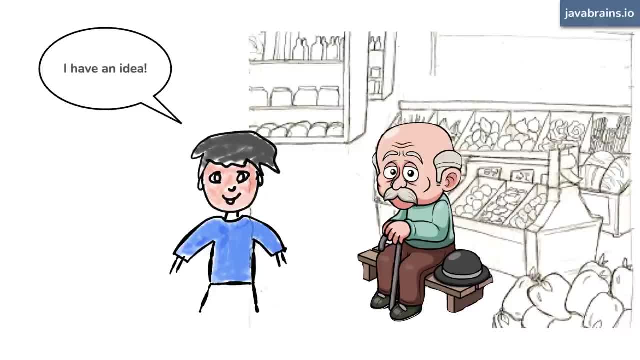 you're taking on so much work managing this big queue of village people, I was thinking I can actually make it easy for you. I have an idea. Would you like to hear it? The old man, while rigid, was also usually nice to the boy, So he said, well, sure, as long as it doesn't change. 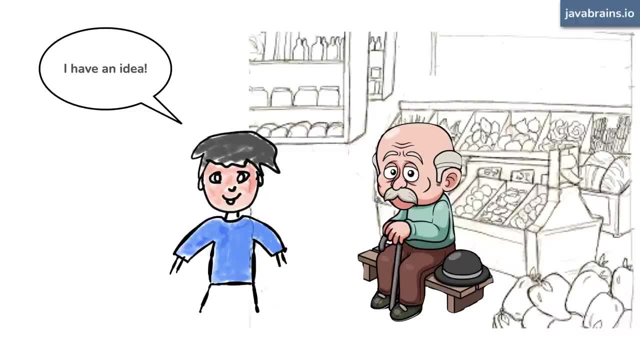 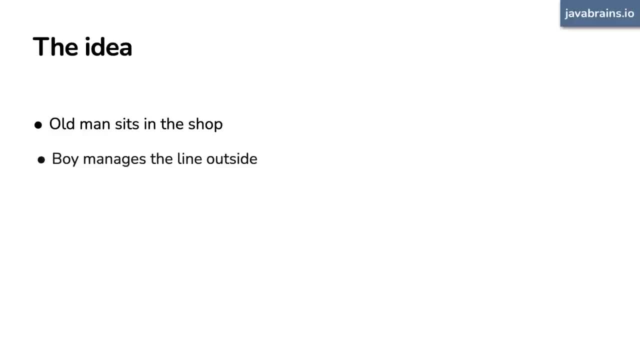 my system. And the boy said: yeah, yeah, yeah, it's not going to change your system. So here's the idea. How about you just sit in your shop and have me let people in one by one? I know you would like your customers in one after another without any gaps. So 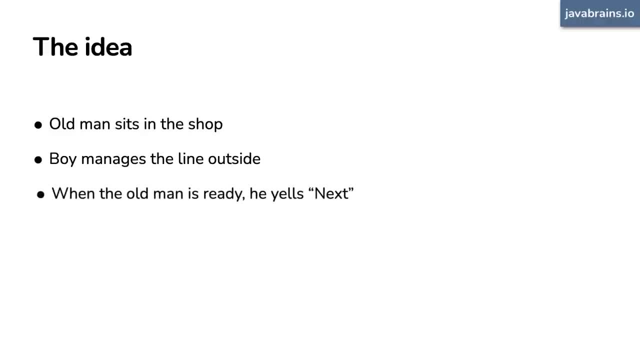 we just take your time And whenever you're ready, you just say next and I'll take care of bringing in the next person in the queue for you. Would you like that? The old man thought about it and felt it was a great idea. So he agrees and said: sure, let's do that. 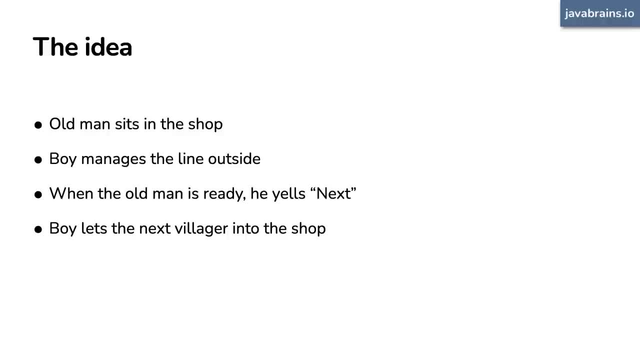 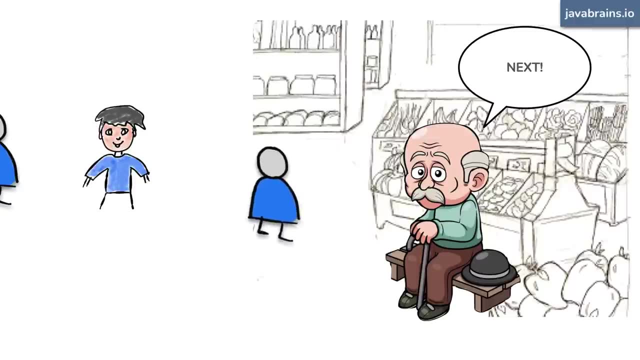 from now on. So the next day, the boy had people stand in line as usual, And when the old man yelled next from inside the shop, the boy had the person at the top of the line walk in, And whenever he was done and ready for the next person, the old man would yell next. 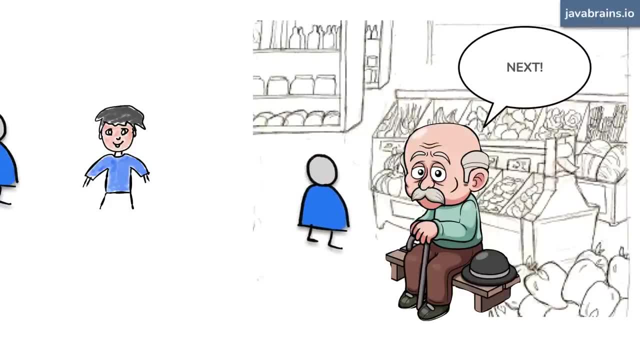 again and the boy would let the next person in the queue, and so on. After doing this for a couple of days and making sure that the old man was happy and it was working fine, the boy gets all of the villagers together and he tells them his plan. They plan together a number based token system. 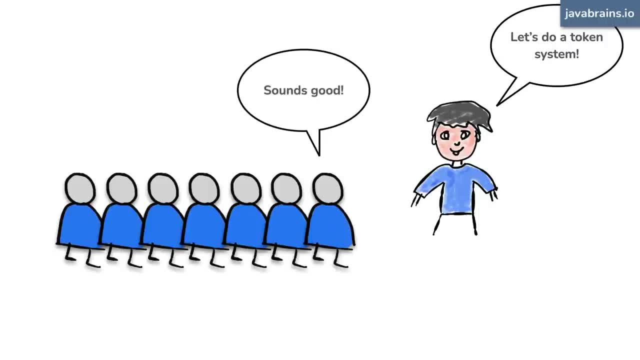 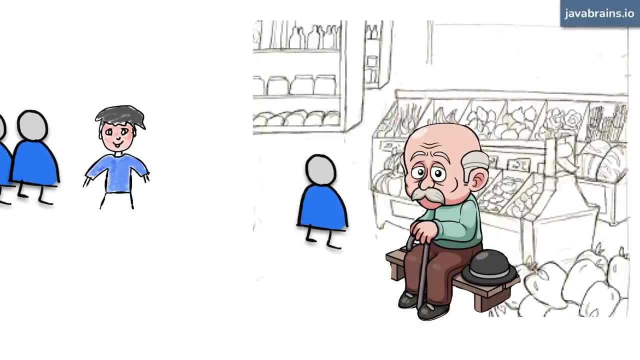 so that everyone can stay at home, except for when it's kind of close to their turn. The plan was settled and put into action the next day. The old man, just like any other day, shouts next when he's ready for the next person. 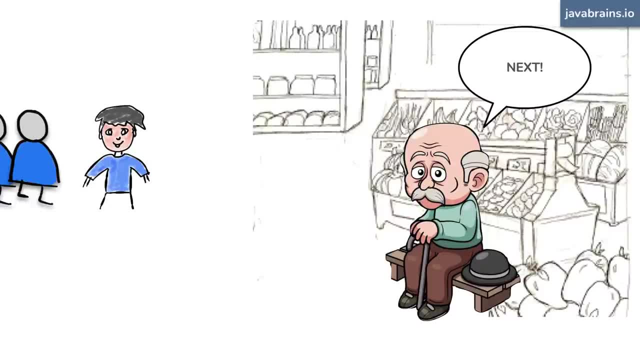 And the boy with the villagers managed to make sure that there is one person walking in when the next call is made. The old man still continues to use the system for recording and serving his customers, But the boy has quietly changed the entire implementation of the system. 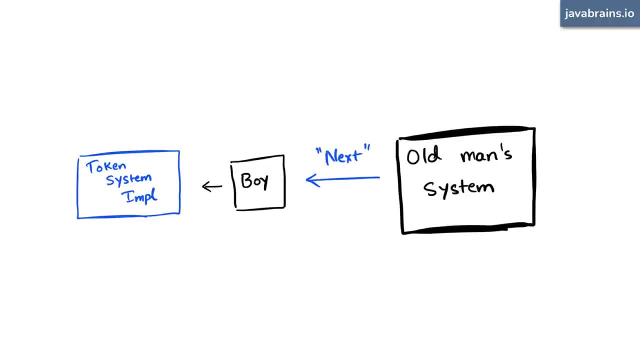 without the old man knowing any of the details. In fact, the contract that the boy has with the old man is so brilliant that the villagers can constantly optimize their system for their convenience, As long as the boy can bring the next person in when the old man yells. 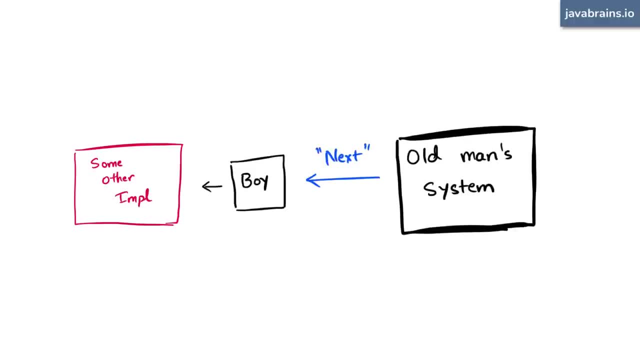 next, the old man's existing system still works, and he won't even know the difference. What the boy and the villagers have come up with is what's referred to in computer science as the iterator pattern. You see the iterator pattern in action in various languages and frameworks. 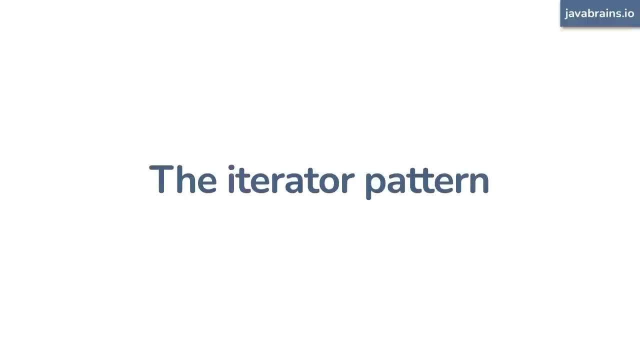 including Java and JavaScript. For example, in Java, we have various different types of collections that we need to deal with in programming. Some collections, like arrays and sets, are sequential. There's an order to them. There are some other collections, like sets. 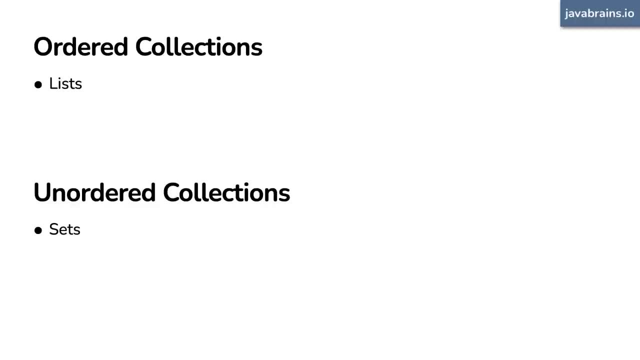 which may not have a specific order to them. This is great, of course, because you want to choose the right data structure for the job. But what happens when you need to loop through every item in a given collection? Well, for a reason, list you need to loop in one way. With sets you need. 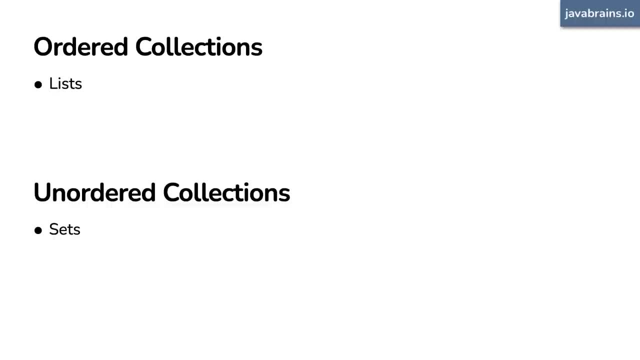 to loop in another way For another collection type. it's something else That's not ideal. Could there be a standard way to iterate over all the elements in a collection without having to worry about how the elements will be integrated into the collection? Well, there are a number of. 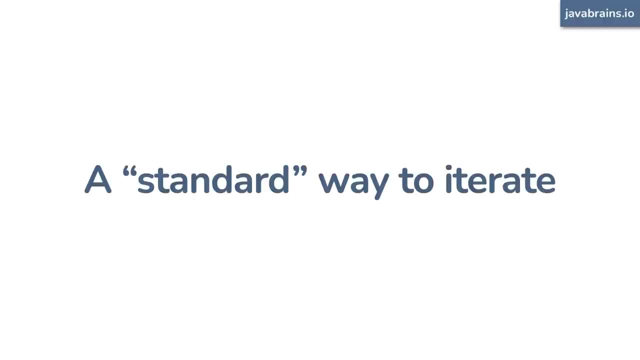 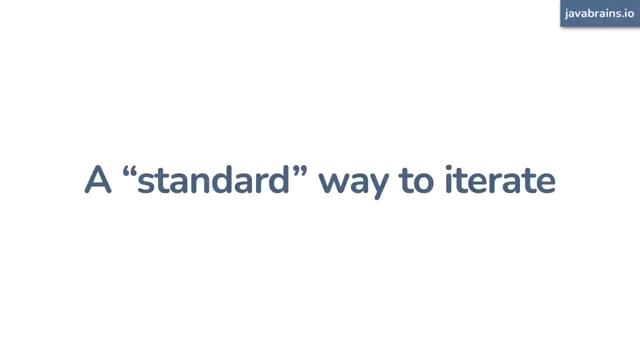 Every different type of collection can come up with a special iterator object. The job of the iterator object is to just have a method that gives you the next object in the collection. It's basically the boy telling the old man: hey, don't worry about the underlying. 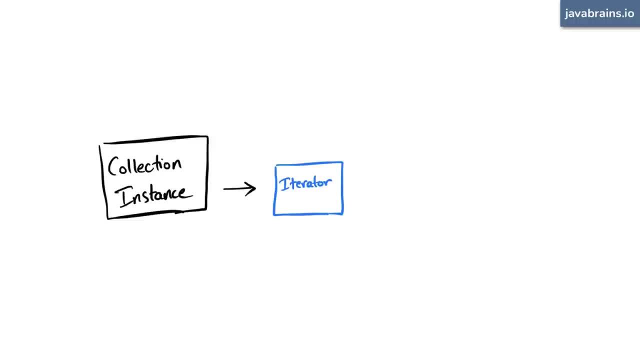 implementation of the collection. All you need at any point of time is just the next element. yeah, So all you need to do to iterate over this collection is just the ability to get the next element And that's it. That's all you need at any point of time. 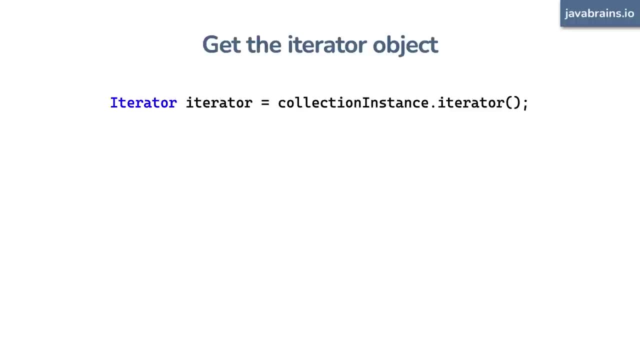 the next element. So the ArrayList has an iterator that knows how to return the next element in the ArrayList. The set has its own iterator that knows how to get the next element in the set. The person calling the iterator doesn't have to care or know what the underlying 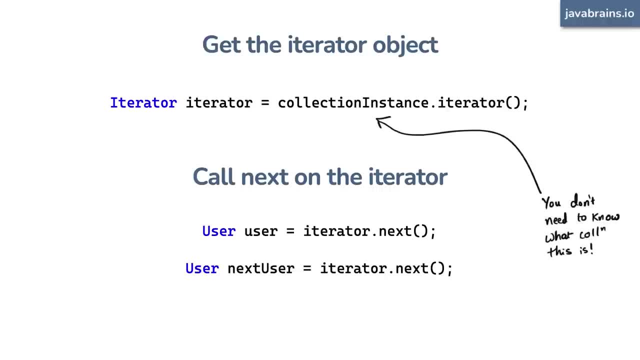 implementation is: If you write code that uses the iterator, you can use that code to iterate on a collection, irrespective of the internal implementation of the collection. JavaScript also has an iterator, which is again an object. with the next method on it, You can create custom. 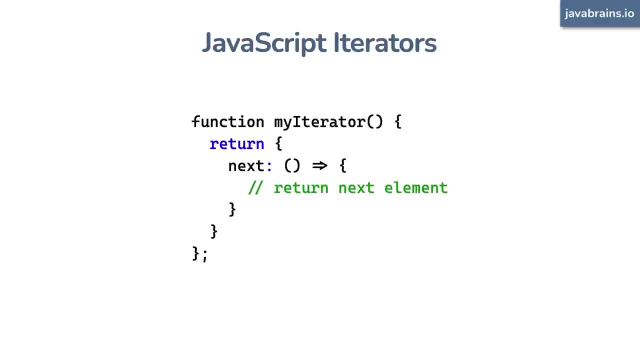 implementations of the iterator that return the next element when the next method is called, whatever the next element happens to be for that particular use case. So this is the basic idea behind the iterator pattern. One last thing you should know is that the iterator pattern also has the ability to signal when the collection is done. 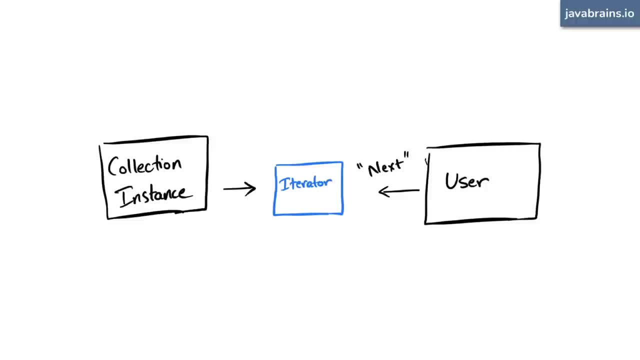 What if somebody keeps calling? next? The iterator needs some way of communicating when there are no more items left. This is done in different ways in different programming languages. The Java iterator has a hasNext method that returns false only when the collection is empty, and it's done. 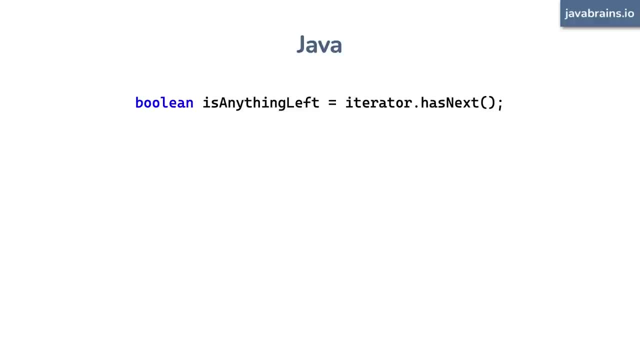 with all the elements. Some other implementations of the iterator pattern, like, for example, JavaScript, returns a done flag, a property on the returned item which, when it's returning the last element of the collection, the done property, will be set to true. However, this is implemented.